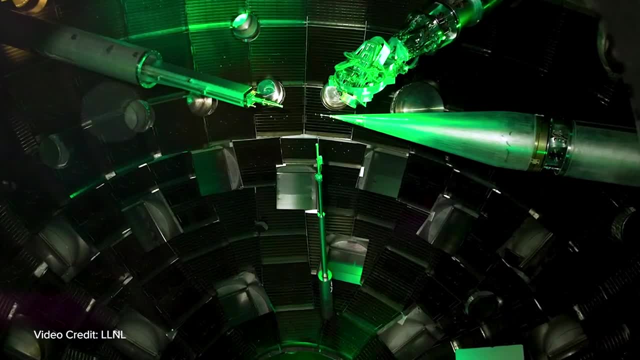 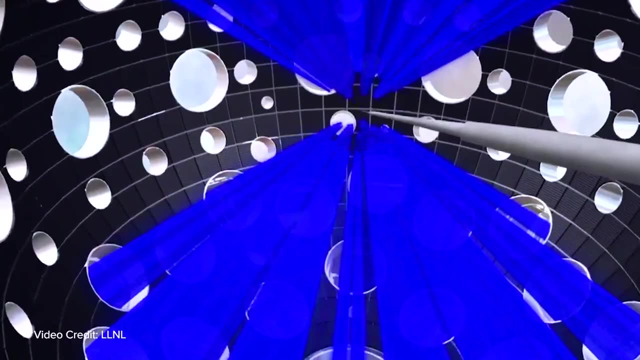 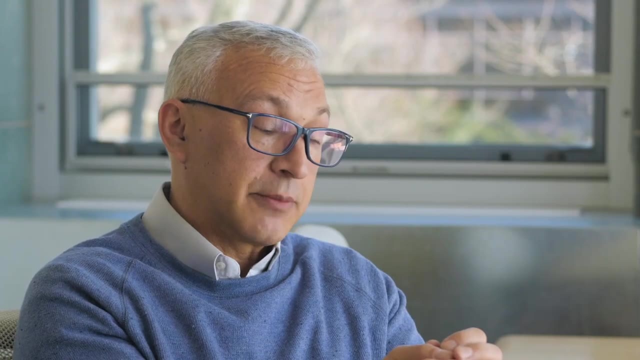 use inertia. So we take a shell of material and accelerate it inwards upon itself, where the fusion fuel is trapped inside. If you accelerate it to high velocities, eventually that kinetic energy that's acquired by accelerating the shell is turned into internal energy. We generate these high pressures and high temperatures, and it naturally wants to blow. 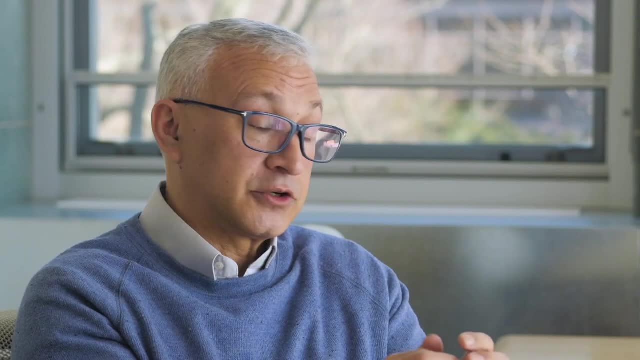 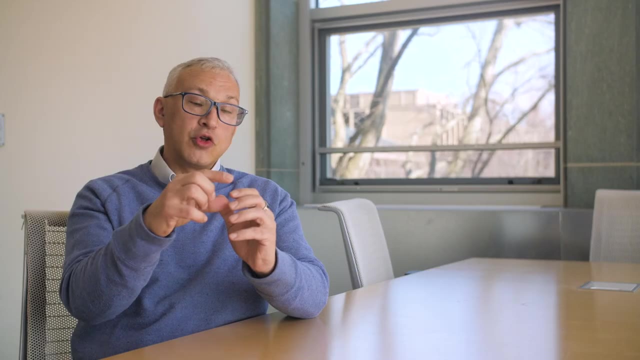 itself apart. Sometimes it's very hard to hold onto something that has a pressure twice that of the center of the sun, But we can hold onto it for a short amount of time. The amount of time we can hold onto it is controlled by, essentially, the inertia of the shell surrounding the hot. 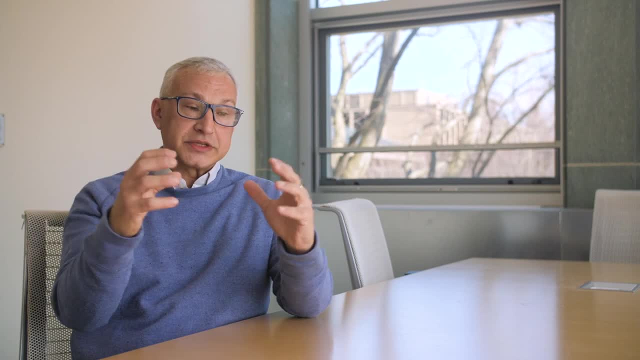 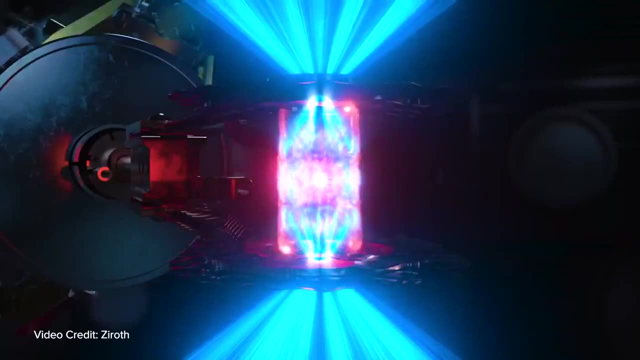 plasma. The idea behind inertial confinement fusion is this acceleration process of a shell and using the inertia of that shell to hold it together long enough for the fusion reactions to take place. but eventually it does blow itself apart. We are a scientific research facility. 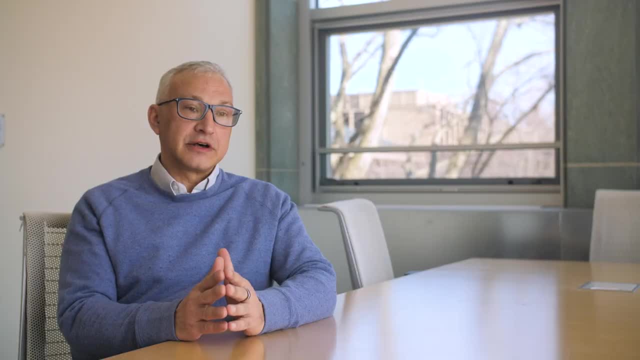 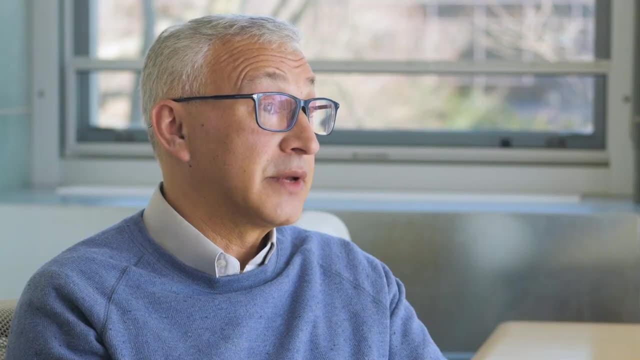 We're trying to prove principles and understand the physics of what's going on. We also have a national security mission involved in the experiments we do For energy production. we have to make the laser a lot more efficient than the one we have now- The national mission. 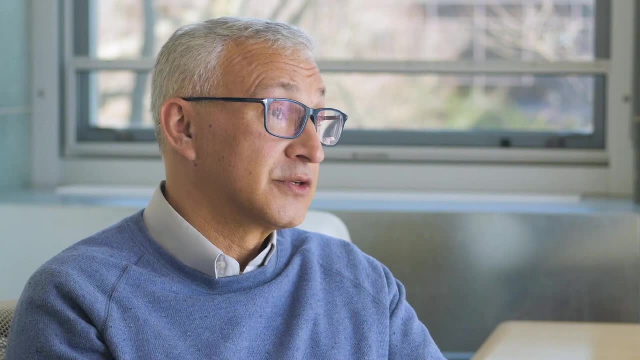 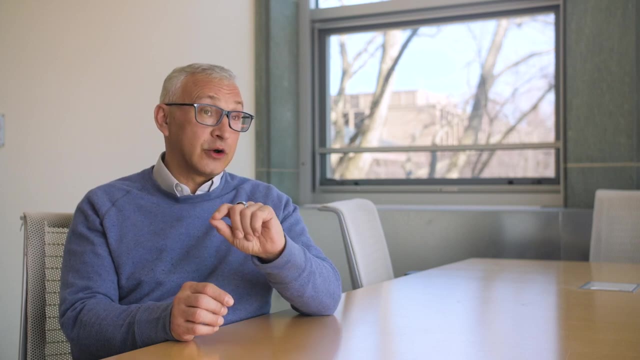 facility, laser, is only about half a percent efficient. So that means of the several hundreds of megajoules of energy that we put into it electrically, we only get about two megajoules out that actually shoot at our target. The other aspects of what will need to be done are the energy production We have to. 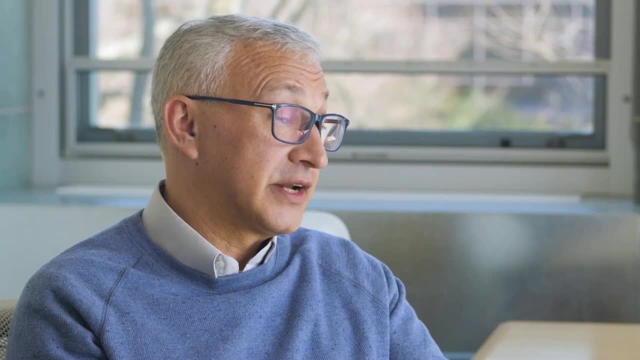 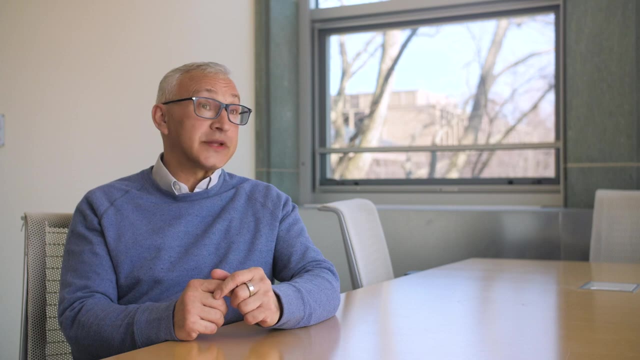 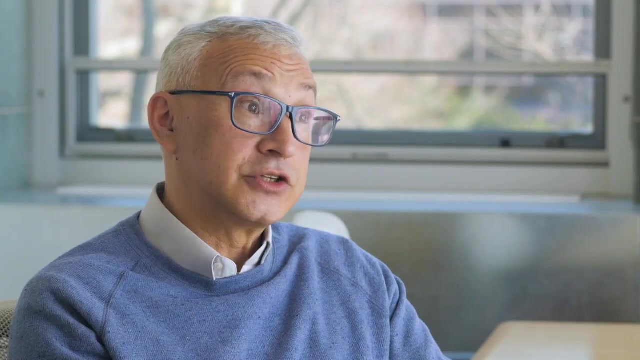 improve the quality of our targets so that they are more robust, less fragile. We also have to be able to do the experiments several times a second. Finally, we have to get a higher gain In order to make up for the laser energy expended to do our experiment. we would. 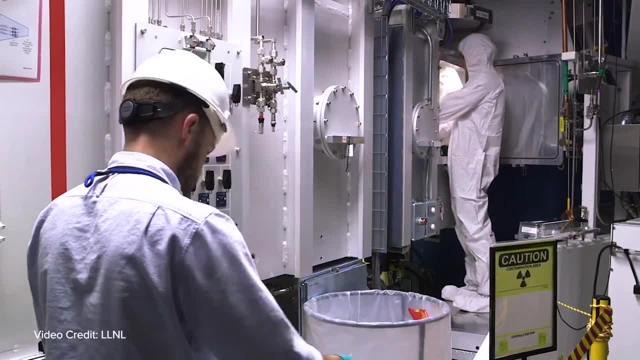 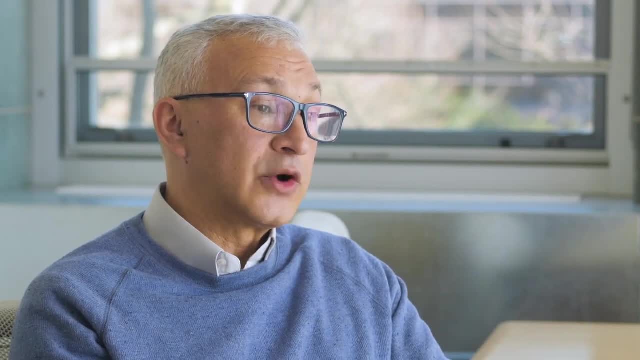 have to increase the gains by at least an order of magnitude. We have to make our implosions more efficient and produce higher yields for the amount of laser energy they put in. One way to do that is creating more compression, where we can squeeze this implosion up down. 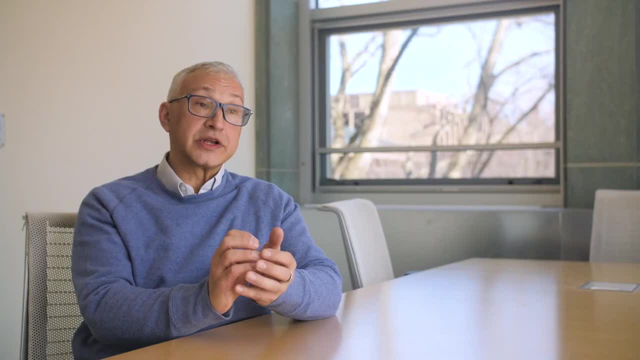 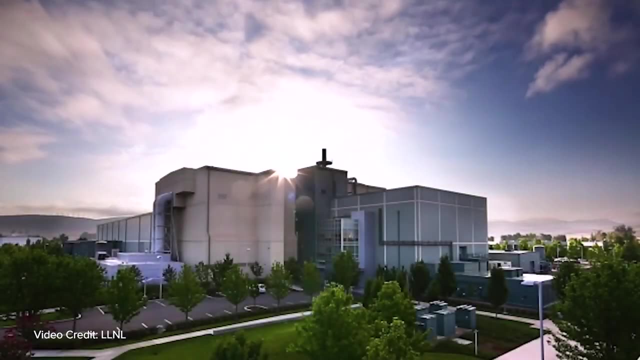 to smaller radii, get the atoms packed closer together so that the fusion reactions are more efficient. I think the future for the field is actually pretty bright. now There are a variety of concepts that need to be explored. I think it is going to turn from a field that is just